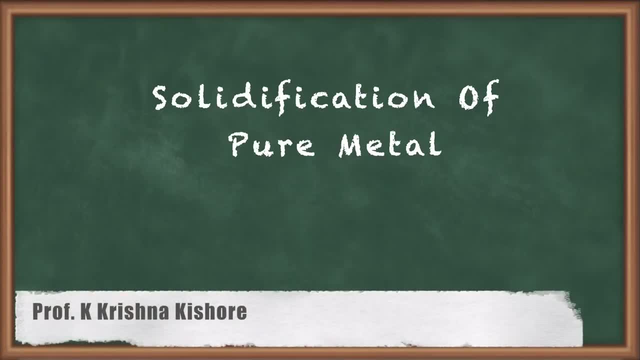 Hello everyone, I am Kakar Lakshmi Kishore, Professor in Mechanical Engineering. Today we are going to discuss solidification of pure metal in material science and technology. So what is pure metal and what is solidification, and what is this solidification of pure metals? All these details we are going to discuss in this video. 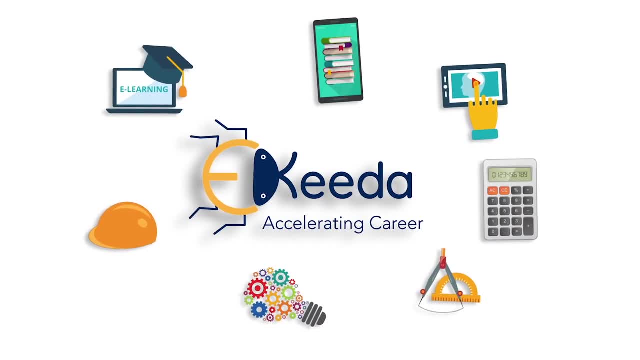 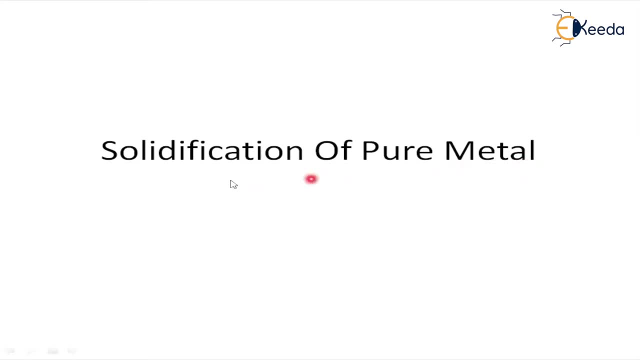 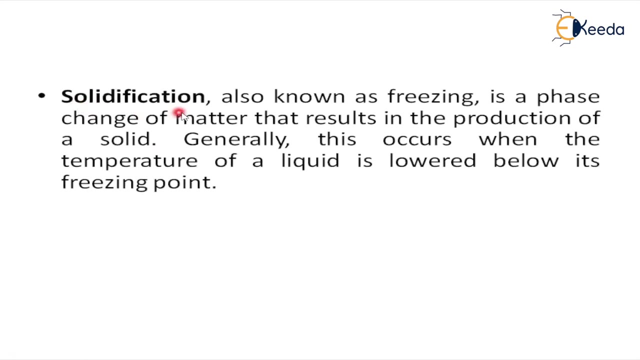 Now let us discuss the solidification of pure metal. Before going to discuss, let me try to give the definition of solidification first. Solidification means- it is also known as freezing- is a phase change of matter that results in the production of a solid. 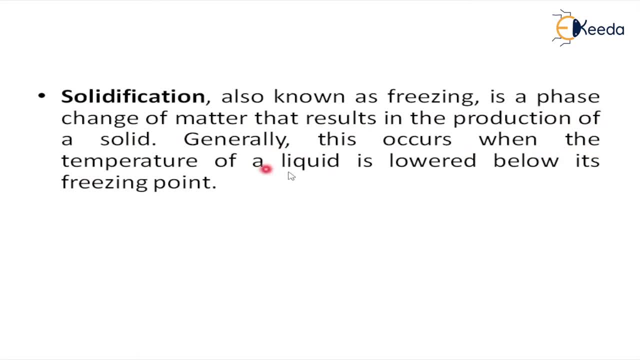 So that means generally this occurs when the temperature of a liquid is high. The liquid is lowered below its freezing point. So that means the liquid is going to become a solid at a particular temperature. That is called as solidification. Now pure metal. What do you mean by pure metals here? 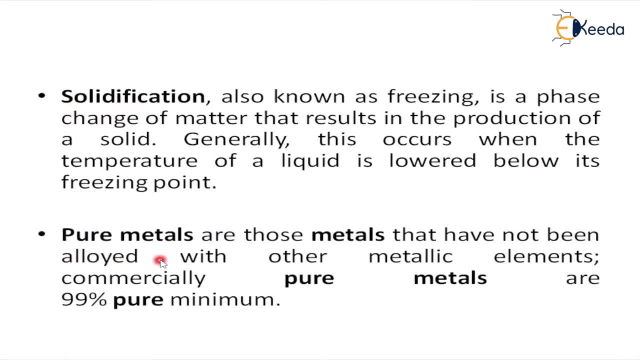 Pure metals means are those metals that have not been alloyed with other metallic elements. This is very, very salient feature. That is important salient feature. Actually, pure metals are 99% pure minimum. We cannot assure that all pure metals are having 100% purity. 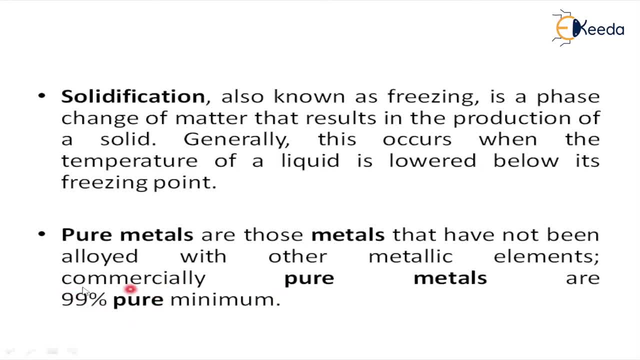 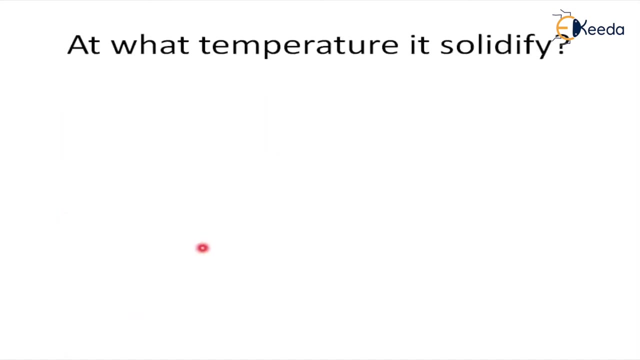 No, we cannot assure like that. We can assure at least 99% purity. The 1% is the other materials Now in that case. so here you have understood the solidification and pure metals. Now, at what temperature it solidifies. So that means at what temperature the pure metal solidifies. 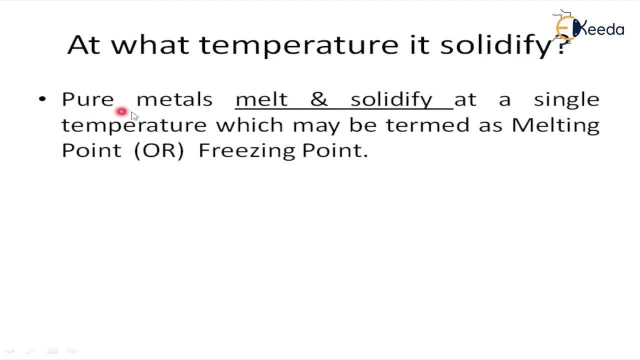 Please observe the sentence first. Here it completely depends on the melt and solidify. That means pure metals melt and solidify at a single temperature, which may be termed as melting point or freezing point. Anyway, we are going to observe this particular temperature. 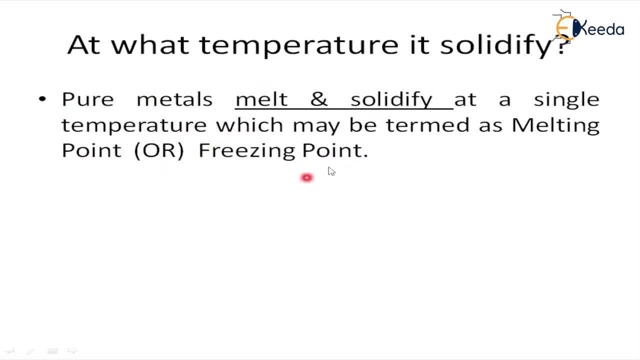 On the graph, which is represented as a cooling curve. So that means here the sentence clearly says that pure metals will solidify at single temperature. So before going to understand the cooling curve, let me discuss what is cooling curve here. The cooling curve means if you observe the cooling curve, the cooling curve means it is a graphical plot of the changes in temperature with time. 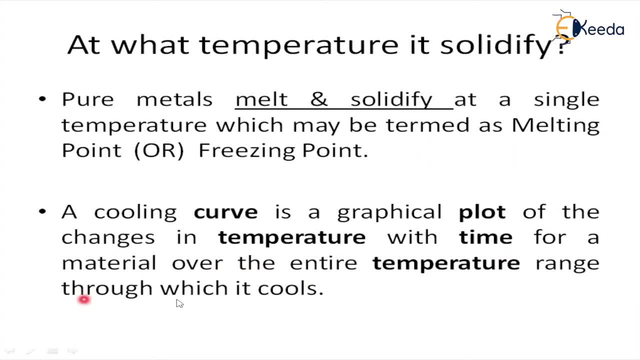 For a material over the entire temperature range through which it cools. So this is only a definition which clearly says that it is a graphical representation and with temperature, Here the temperature is important. That means temperature versus time. So temperature is on y-axis, time is on x-axis. 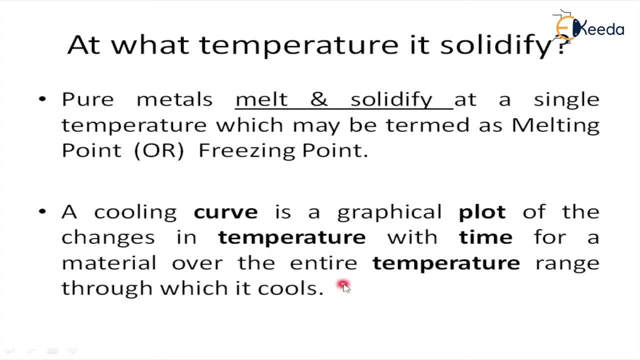 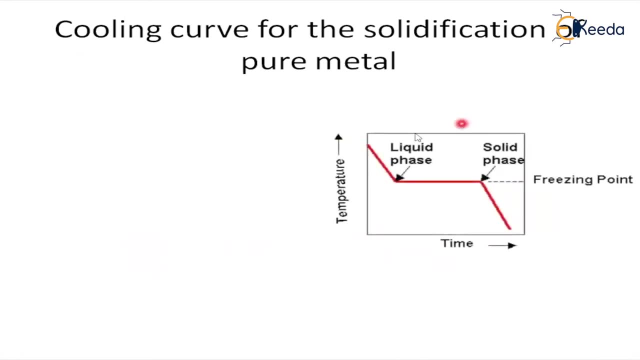 And at the various temperatures, how the material behaves. All these things, all these data are going to be noted down, Noted down in a graphical plot. So let us see the cooling curve for the pure metal. Please observe the cooling curve for pure metal. 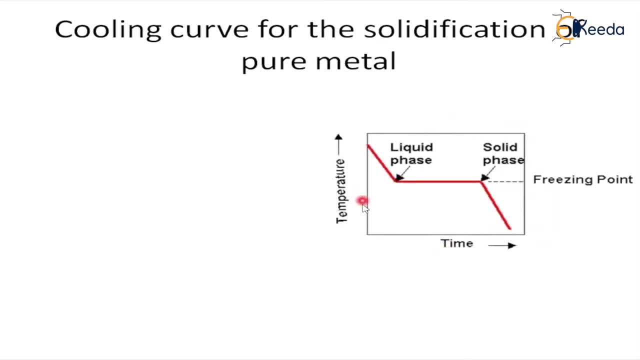 This is the cooling curve for pure metal. So that means if it is not pure, if the alloys are existed, then the phase, that is, this diagram, the cooling curve diagram, may have some changes If you observe the red line here in initial stage. 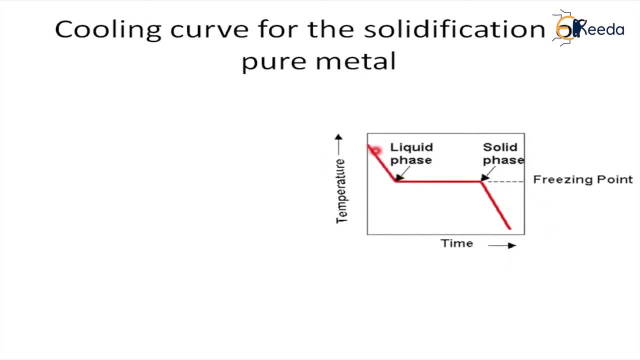 So that means at initial time it is the liquid phase here And up to some position This is the liquid end point At this point. so this is called as a freezing point. So that means solidification starting point. If you observe this here, for pure metal this solidification temperature is a horizontal line. 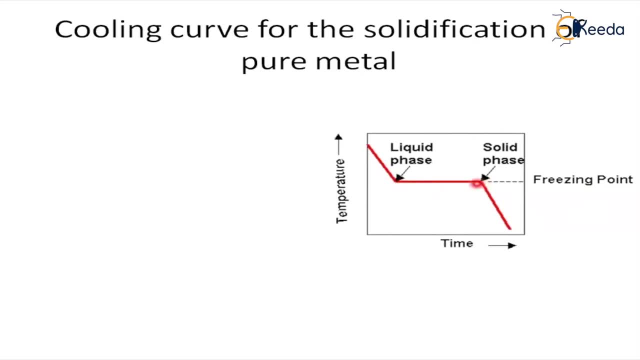 If solidification temperature is a horizontal line, it means that the temperature is constant. That means at constant temperature or at the constant freezing temperature. the solidification is happened for pure metal. This is the solidification ending point here. That is after that. that means almost the total liquid is going to be disappeared after this point. 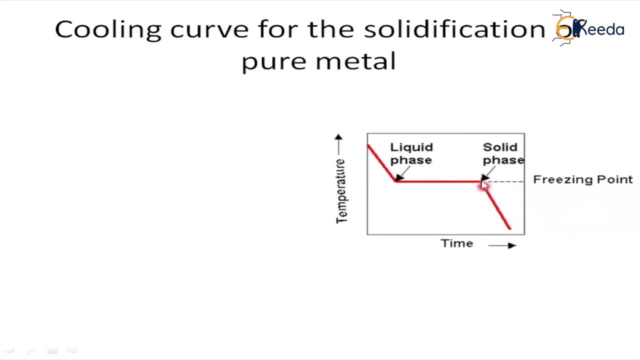 Then all this is a solid state. All this is solid state. So this is for pure metal. If you observe this under equilibrium conditions- here the important parameter is- this particular graph may be valid. That is, we can validate this graph if the conditions are equilibrium. 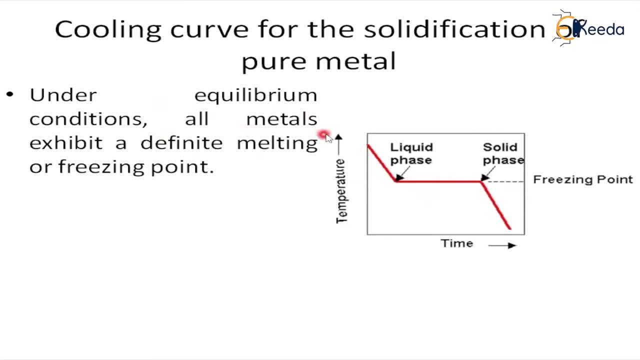 All metals, whatever the metals which are in periodic table, all those metals will exhibit a definite melting or freezing point here. So that means here this pure metal, whatever the pure metal, that is 99% purity, this metal cooling cow will show a horizontal line at the melting point or freezing temperature. 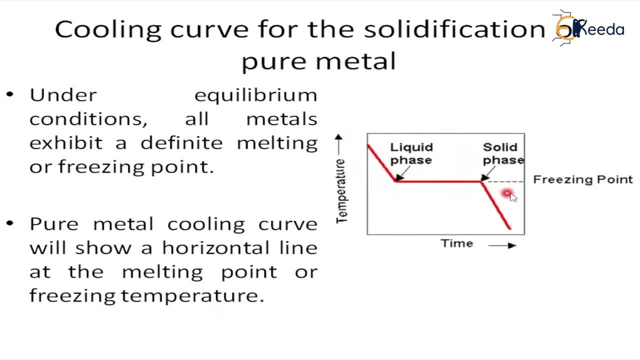 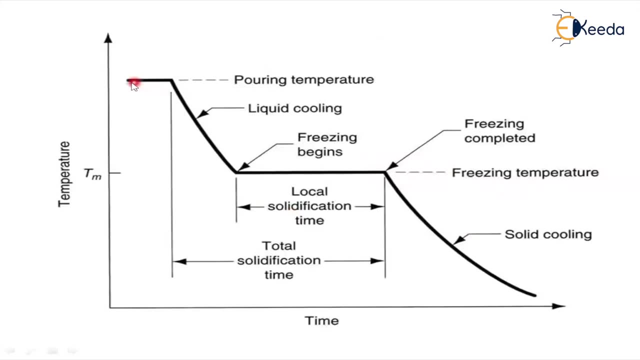 So that means this is also represented as a melting point or freezing temperature or freezing point. Now let us observe the various features and various points in cooling cow, that is for pure metal. If you observe here, this is the detailed graph between temperature versus time for pure metal. 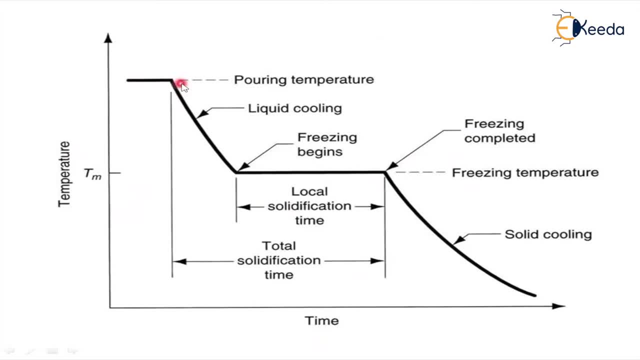 So this is the pouring temperature. That is, at the initial stage at which the hot metal enters into the mould cavity and after it settles down. So this is called as a pouring temperature. After that it is in liquid state. Slowly, the liquid is going to be cooled. 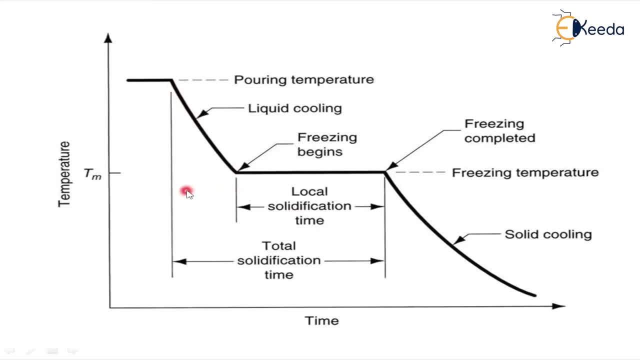 That means this is a liquid cooling. This is the time. It will take some time for cooling. So all this, in all this state, the metal is in the form of liquid, That is a hot metal And at some position the freezing begins. 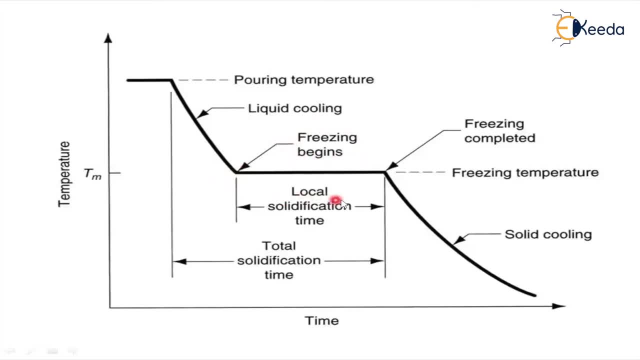 That means solidification starts, which is also represented as a local solidification time. So that means, what do you mean by local solidification time? Local solidification time means the freezing starting temperature to the time between freezing starting temperature to the time at which the freezing is completed. 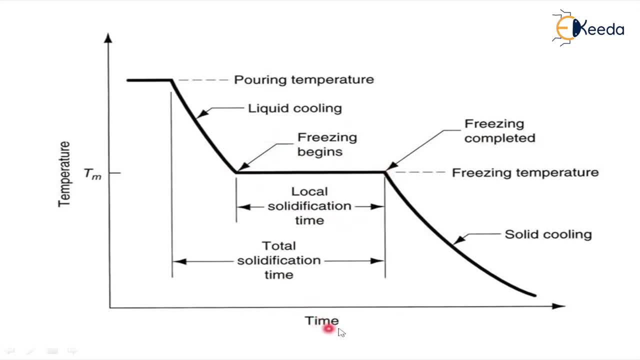 So that means between these two points, whatever the time is existed that is called as local solidification time And total solidification time. here we also consider total solidification time. Total solidification time means at which after pouring is completed. 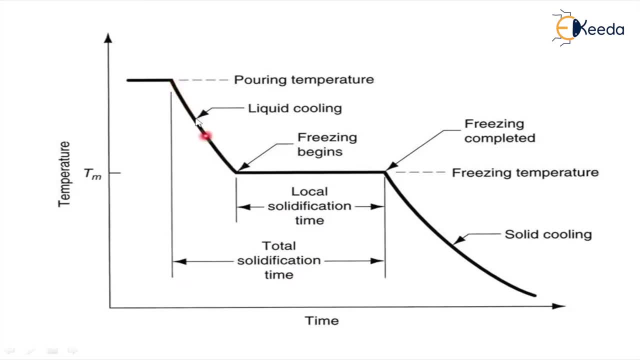 now the liquid is going to be cooled, If you consider this also as a solidification time. so this is liquid solidification, this is solid solidification. If you add these two, then that is represented as total solidification time Now, after that. 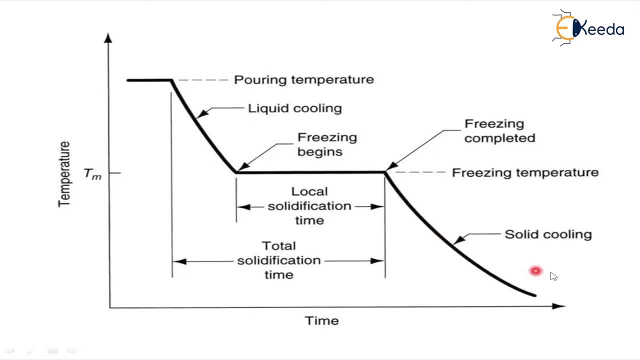 as we have seen the last one, that is, in the last image, the same picture, but this is a detailed image. This is called as a solid cooling time. It will be in the form of a curve, slowly. It will cool slowly, the solid. 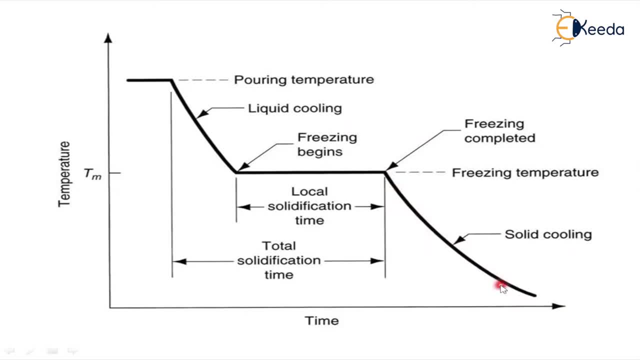 After that it will completely converted as a solid form, And here two conditions may be existed. So that means this type of horizontal line. you are observing the cooling curve, freezing temperature, as a horizontal line. This horizontal line is completely depends on the condition. 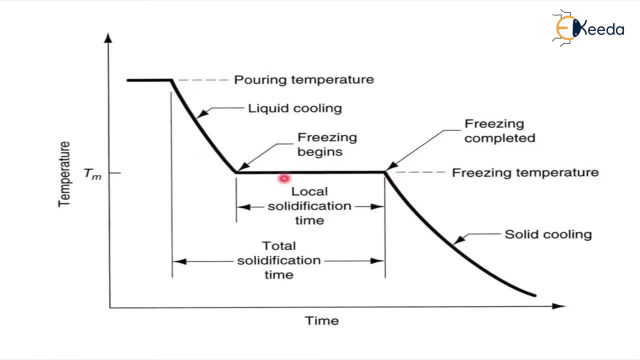 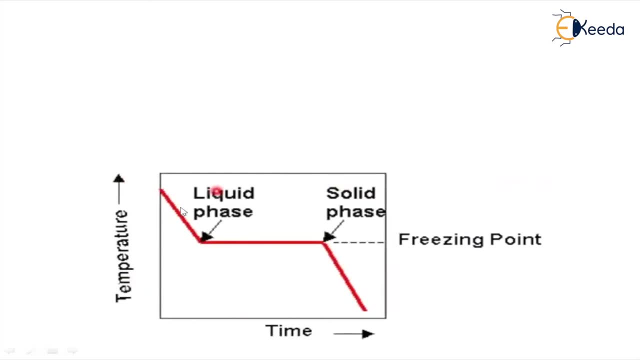 Now let us see on what condition the horizontal line depends. Now see the first condition here. Already, you have seen this image. When is this image going to be formed? So that means when the horizontal line is going to be formed. 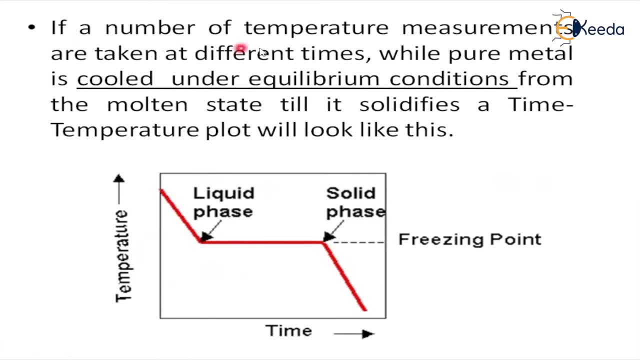 Please observe the sentence here: If a number of temperature measurements are taken at different times while pure metal is cooled under equilibrium conditions, Here the condition is if- whatever the discussion up to now, that is, we have discussed- if it comes under, if it is cooled under equilibrium conditions, then we can say that this type of phase diagram. 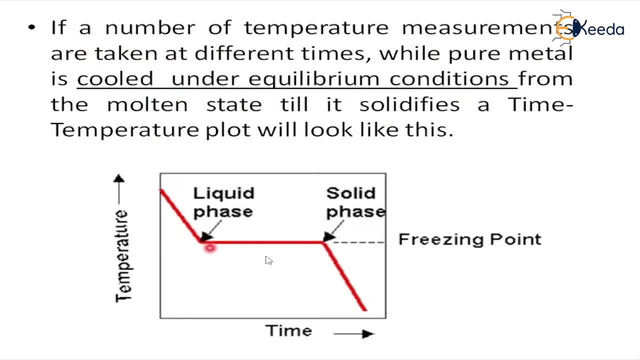 So that means a horizontal Line for solidification is going to be formed and the condition is from molten state till to solidifies a time temperature plot. So this is also represented as a time temperature plot. So that means graph will look like this: 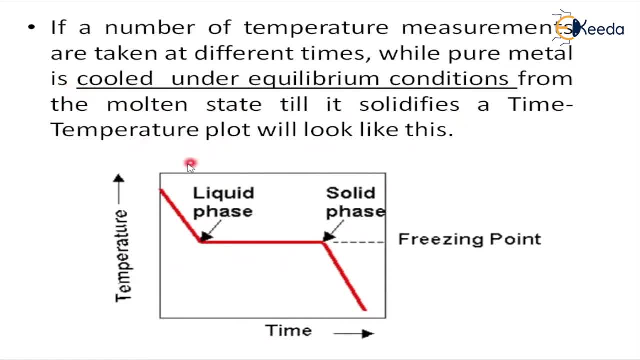 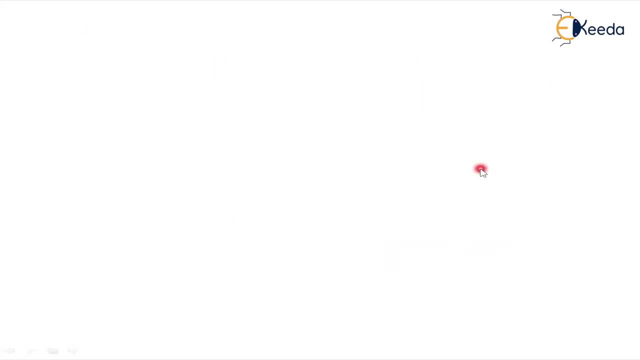 Here the condition is for a horizontal line to be formed is cooled under equilibrium conditions. So let us see the second condition here Now Observe this image. this is also cooling curve for pure metal, but if you observe here, this type of a small curve may be formed for some times instead of cooling curve. 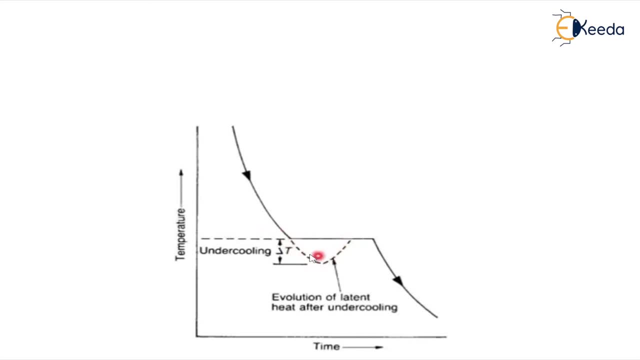 So that means only as portion. a portion of the horizontal line may be formed like this When this is going to be formed, Please observe the sentence here: Here- if a pure metal cools rapidly. So this is the main point here. 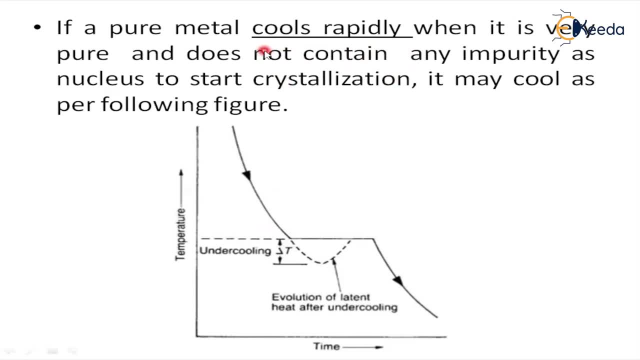 When compared to the previous case. the previous image shows that it forms under or it cools under equilibrium conditions. But here, if it cools rapidly, when it is very easy, or when it is very pure and does not contain any impurity as nucleus to start crystallization, it may cool. as for the following figure, 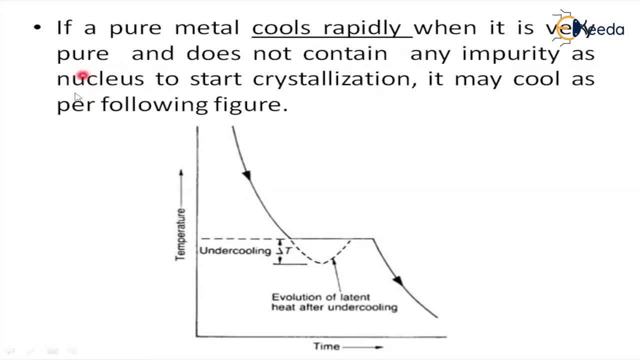 Here two sentences that we have used. One is a nucleus here, And what is this? This is called as under cooling Here, nucleus. what do you mean by nucleus and when it is going to be formed, and what do you mean by under cooling? 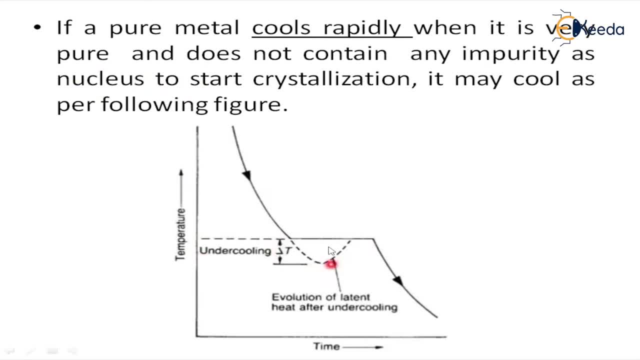 Let us discuss the under cooling and nucleus. Before going to that, let me clear. this type of under cooling will be happened when the metal cools rapidly, and this under cooling may not be formed if this metal is cooled in equilibrium conditions. That is the main point. 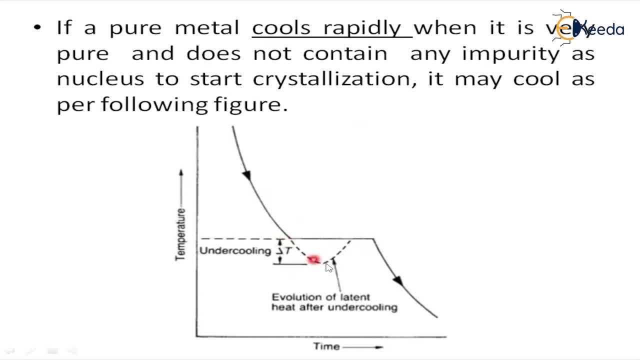 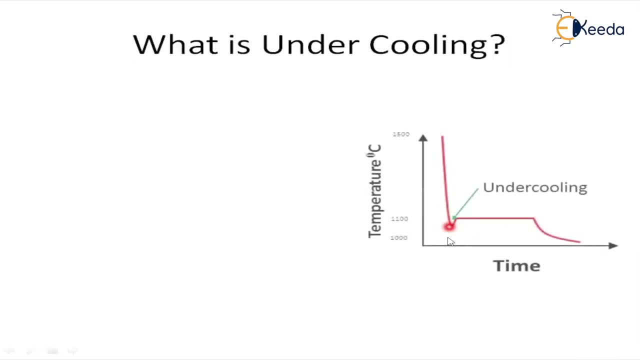 That is the main difference between before- that is, without under cooling- and with under cooling. So let us discuss what is under cooling here. Observe the image. Only a small portion on the horizontal line is formed as a crust like this. That means this area is represented as an under cooling. 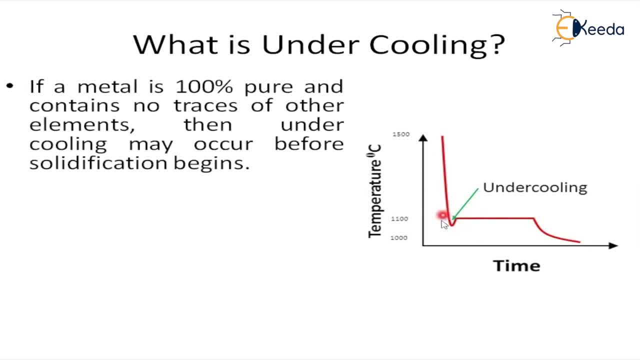 And if, if the suppose if a metal is hundred percent pure and contains no other traces, And if the suppose if a metal is hundred percent pure and contains no other traces of other elements, then under cooling may occur before solidification begins. here this at this: 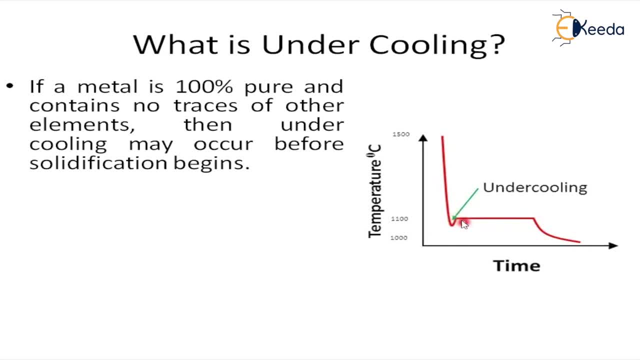 point. this is the solidification point here. before this solidification begins, this type of under cooling maybe happens if it is 100 pure but which is not existed in this universe. so that means almost all metals are considered as 99 purity. so that means for all the pure metal we are going to 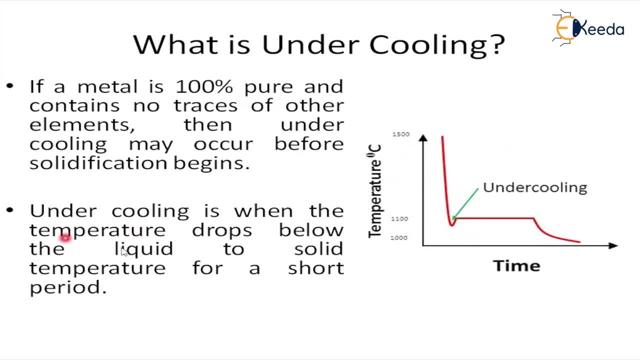 get this type of only under cooling is when the temperature drops below the liquid, below the liquid to solid temperature, for a short period only. so he observed this word here. this only happened for a short period, so that may say not that, not the much time here that. 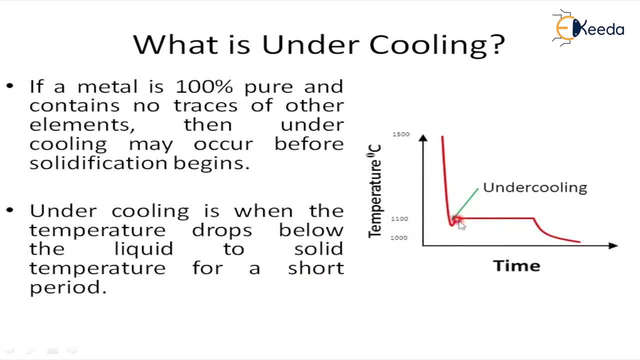 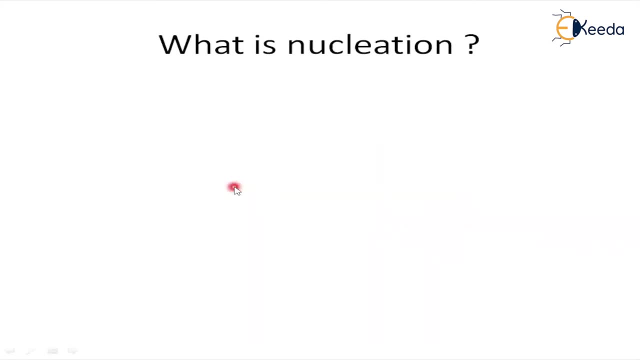 means only for a shorter period of time. this wonder. cooling is happening and again the freezing temperature starts and the freezing temperature ends as a straight line. so this is about under cooling. then what is nucleation in solidification of pure metal? observe the nucleation here, observe the microstructure image in initial stage that 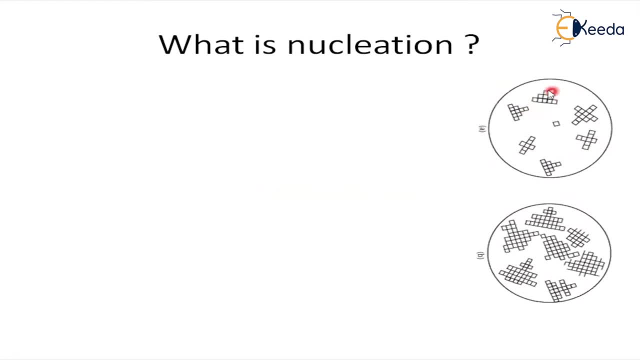 means when metal is going to be cooled, then these type of crystals, all these type of crystals, that is, the single crystals, are going to be combined like this. so that means at the solidification temperature, atoms from the liquid. so all these are liquid atoms here, such as molten. 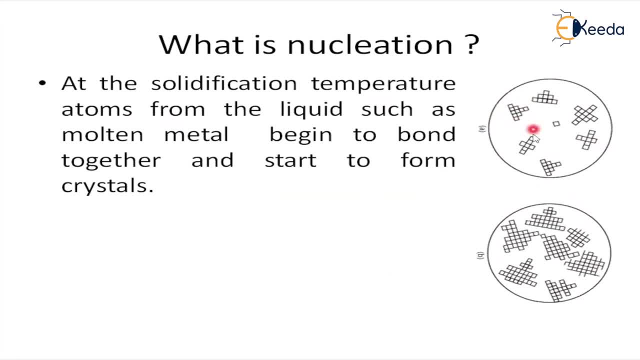 metal, that is when it is at molten condition, begins to bond together and start to form crystals. this momentum, whenever they want to begin to start or bond, to start or bond together, then we can say that the moment a crystal begins to grow is known as nucleus. 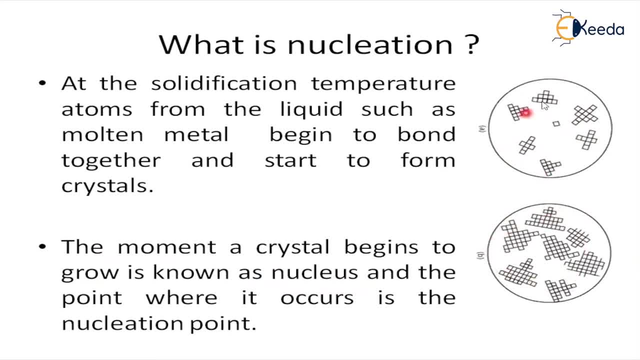 and you can see the nucleus formation here. slowly all these, these two combine together and form a single one and this is called nucleus and the point where it occurs is the nucleation point at which this particular nucleus is observed. this is called as nucleus and nucleus point here and how they are growing. here you can observe the 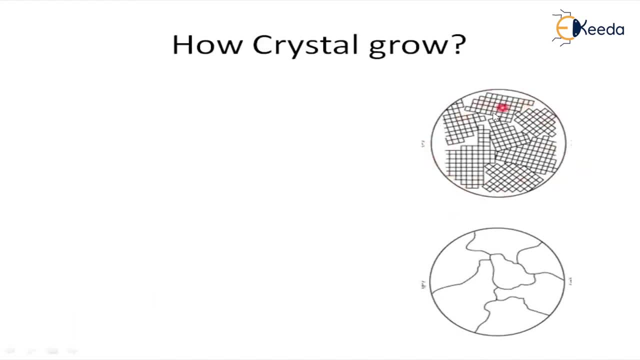 continuation images here. in the earlier images they are about to bond. here they are born completely here. if you can observe the sentence here, when the metal begins to solidify the multiple crystals- so all these are multiple crystals, only all these are multiple crystals- begins to grow in the liquid,